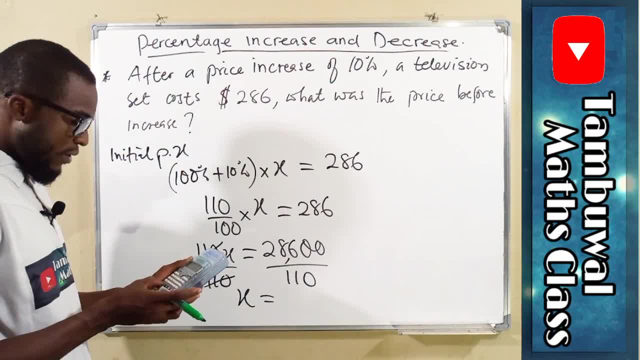 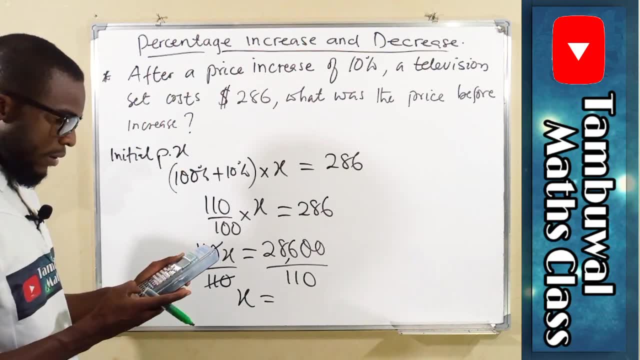 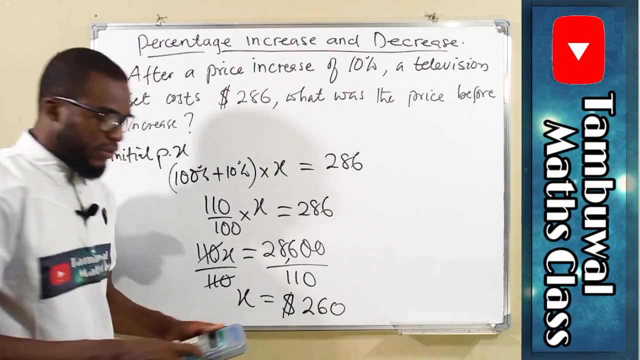 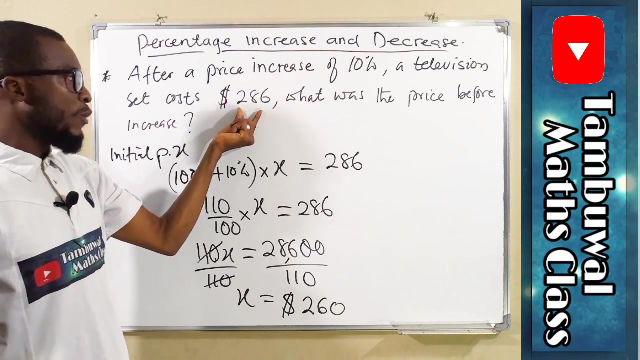 And finally, X is equal to 28,600 divided by 110.. And we have $260.. $260.. So this was the initial amount, before it was increased by 10% to result to $286.. Let us look on to another question. 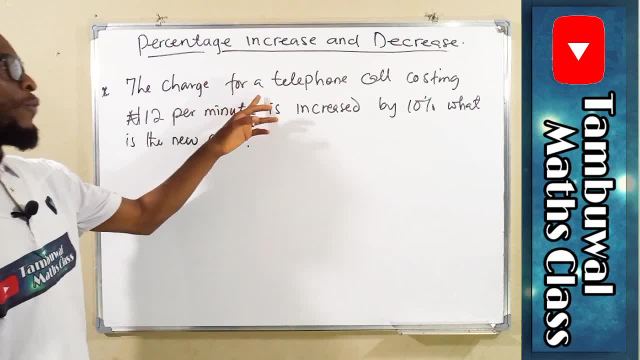 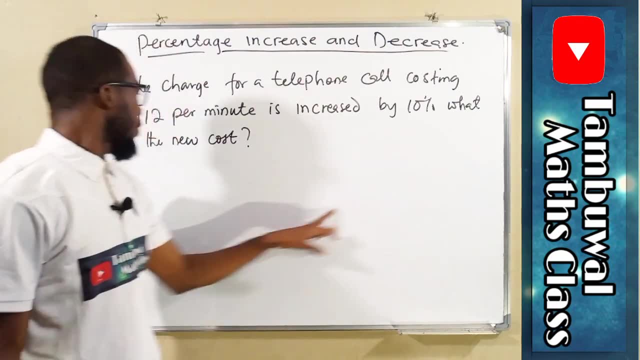 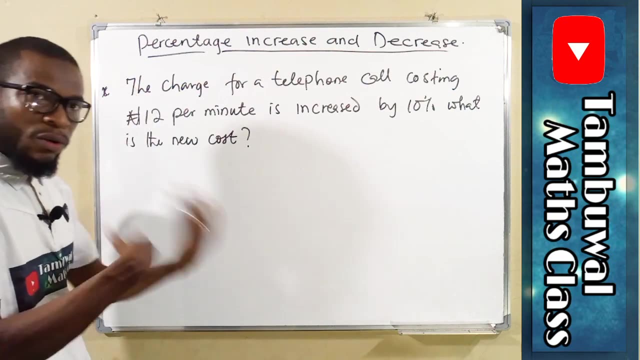 This question says the charge for a telephone call costing 12 naira per minute is increased by 10%. What is the new cost? Initially, this is what is charged per minute- 12 naira- And later on increased by 10%. 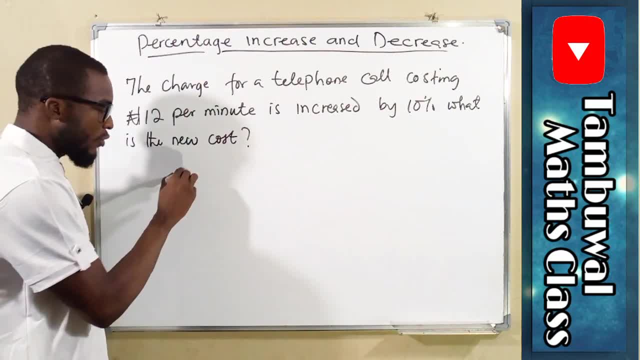 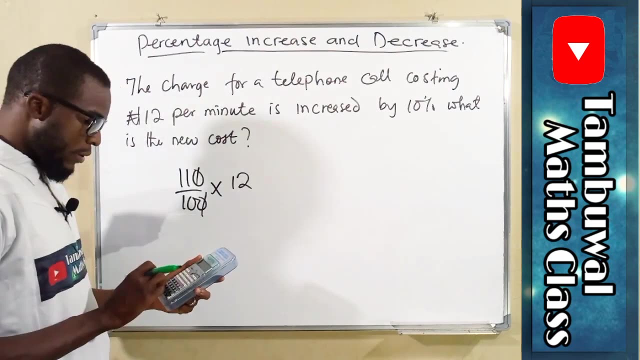 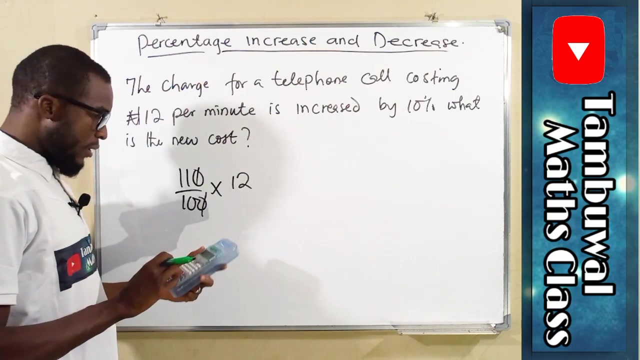 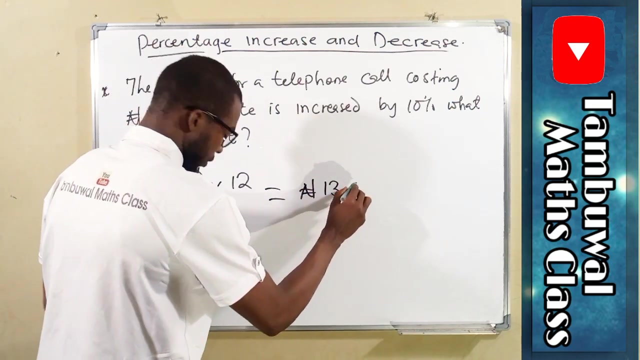 We want to find the new cost, So we have 110 collectively out of 100 times 12.. This will cancel this. All we have is 11 times 12 divided by 10.. 11 times 12 is 132.. Divided by 10 will give us 13 naira to couple. 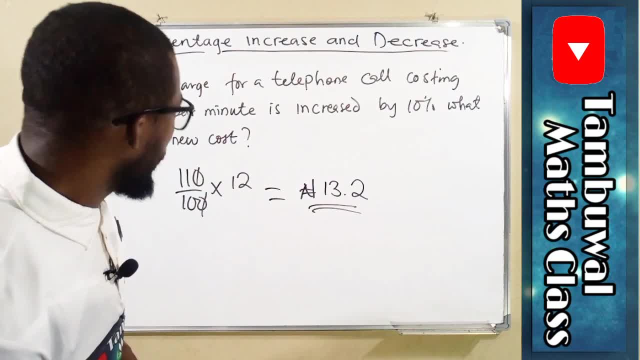 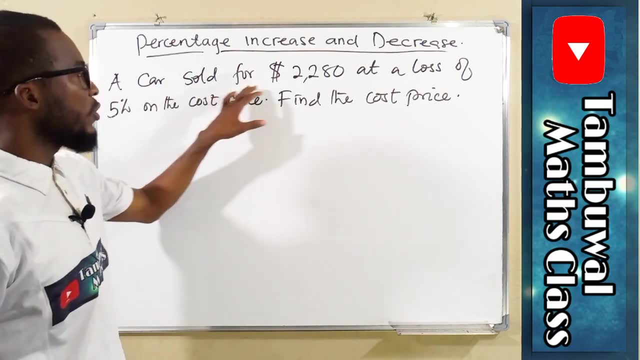 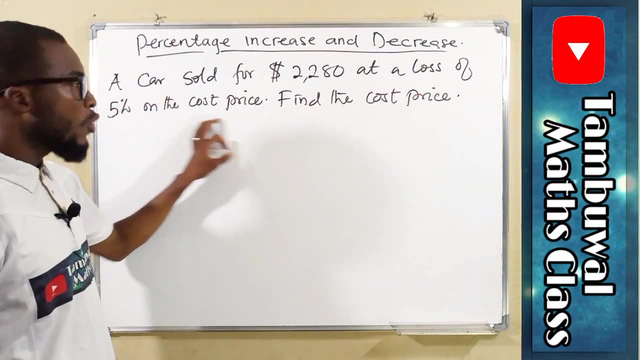 So this is the new amount per minute. Now let us look on to the last question. The last question says a car sold for $2,280 at a loss of 5% On the cost price. we actually find the cost price, Since there is a loss. 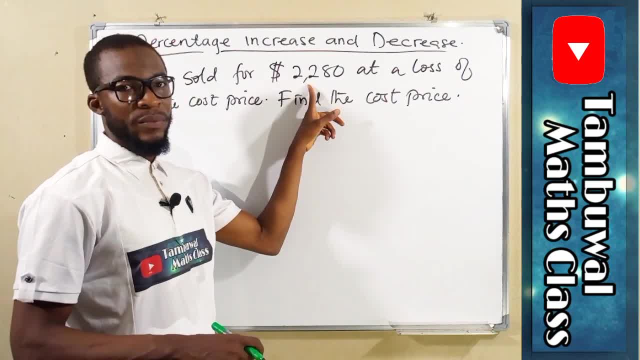 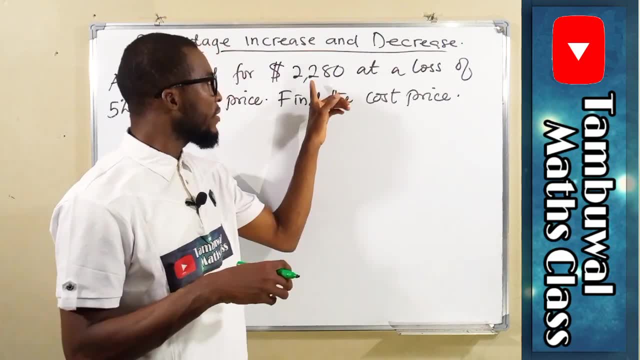 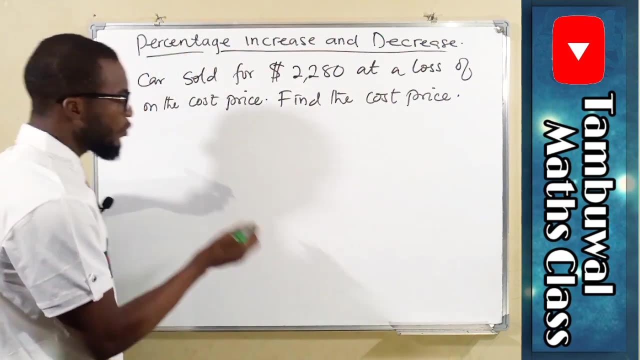 it means that the cost price is higher than the selling price And 5% of the initial price, which is the cost price, was removed from that cost price to rise to this current amount, which is the selling price. So we don't know the cost price. 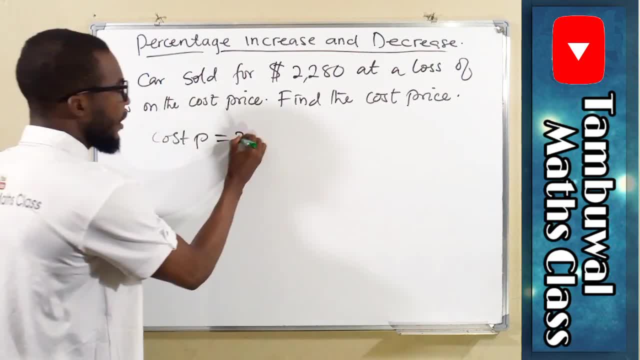 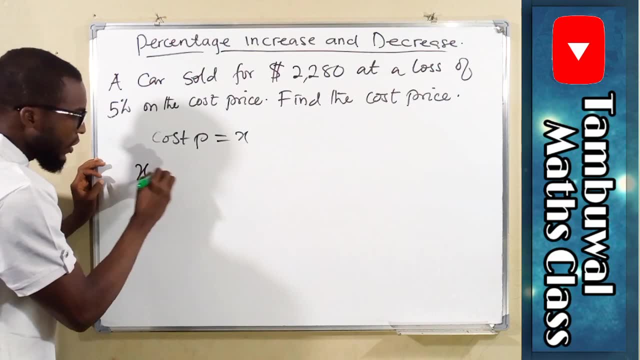 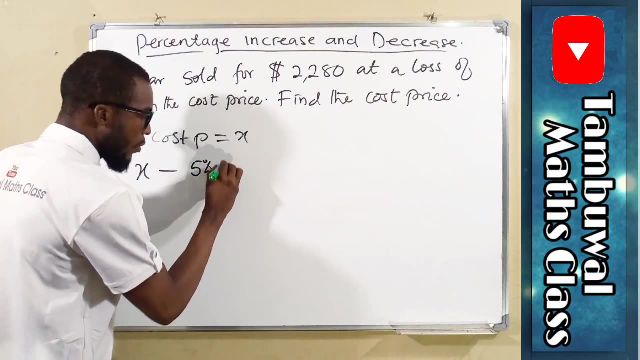 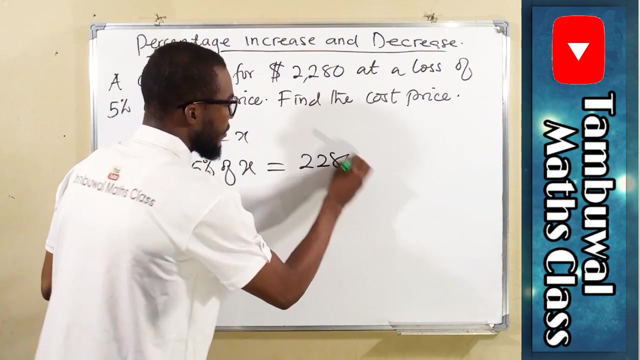 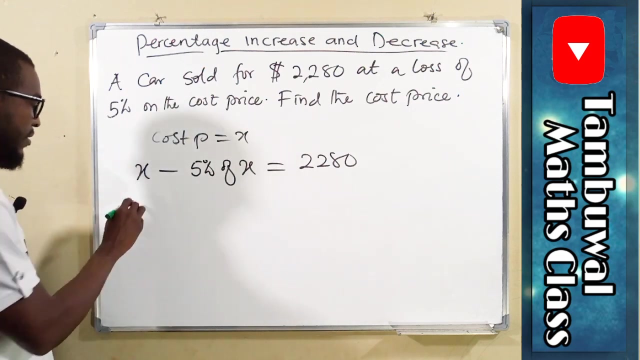 We can let it to be equal to x. This is the current amount. This is the original price, which is x. Subtract 5% of that amount to get rise to $2,280.. This can be seen as 100%. Yes, this is 100%. 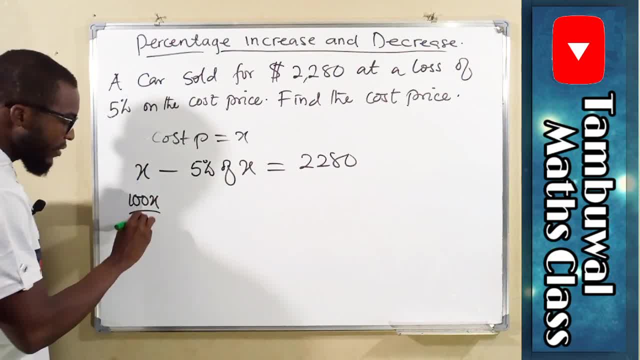 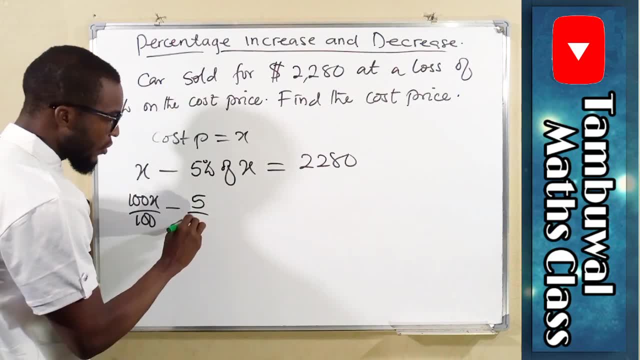 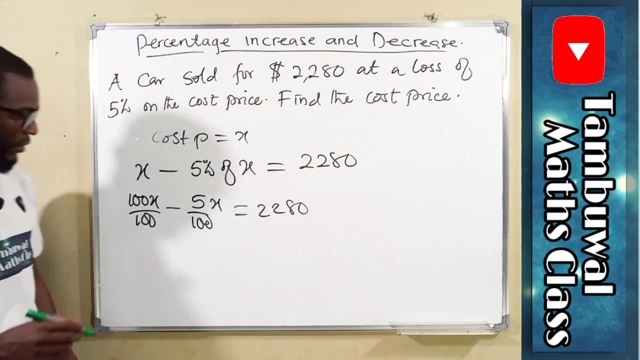 So this is 100.. x over 100 minus 5% of x is the same thing as 5 out of 100 of x, And this is equal to $2,280.. The denominators are the same, So this minus this is equal to 95.. 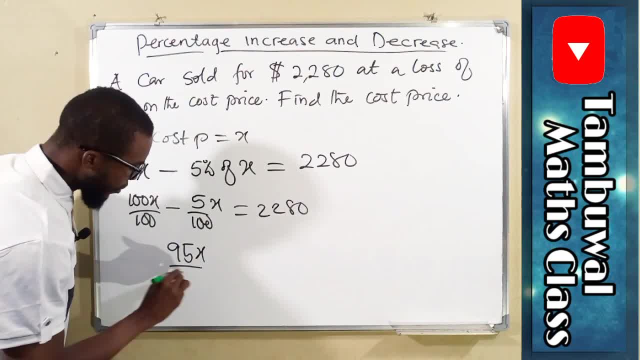 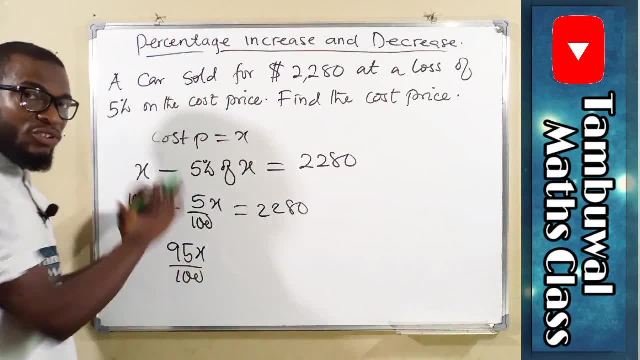 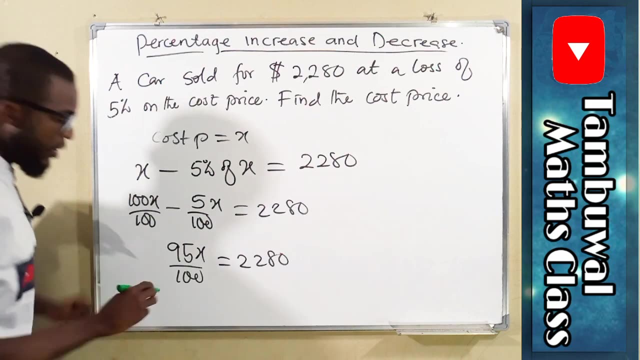 We have 95x over 100.. Remember, this is percentage decrease. 100 minus 5 is the same thing as 95.. This is just another approach. This is equal to $2,280.. We can multiply both sides by 100.. 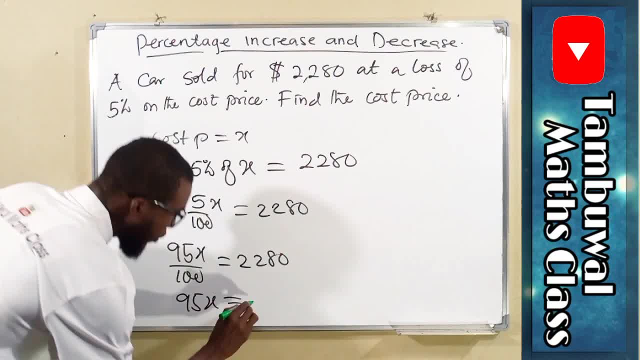 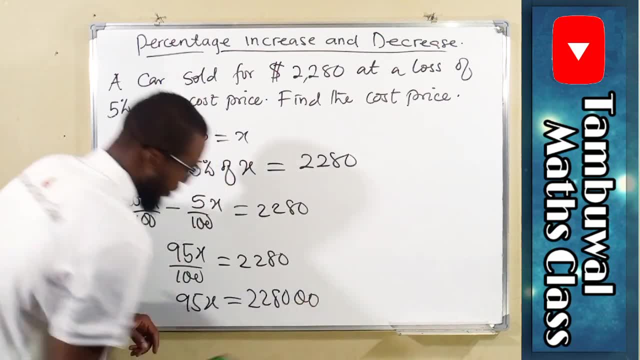 We have 95x here equals. We add two zeros. here We have 2, 2,, 8,, 0.. Then these other zeros. To find the value of x, which is the cost price, we divide both sides by 95.. 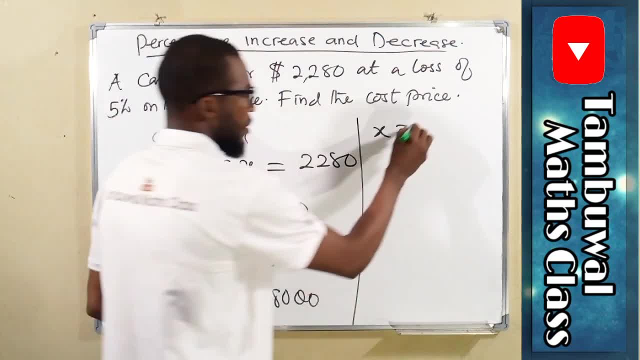 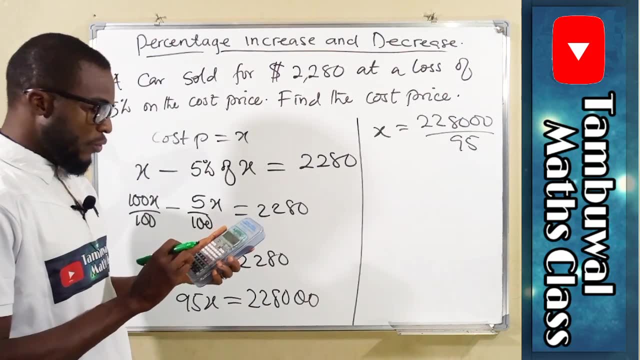 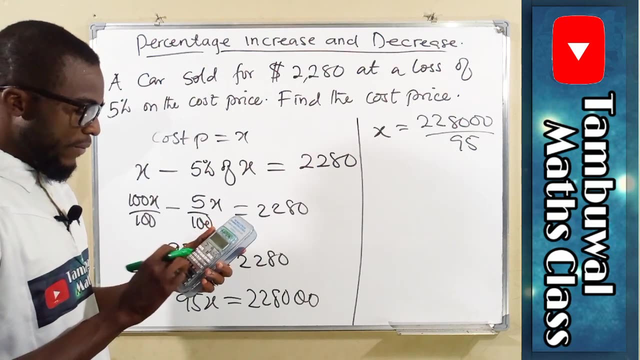 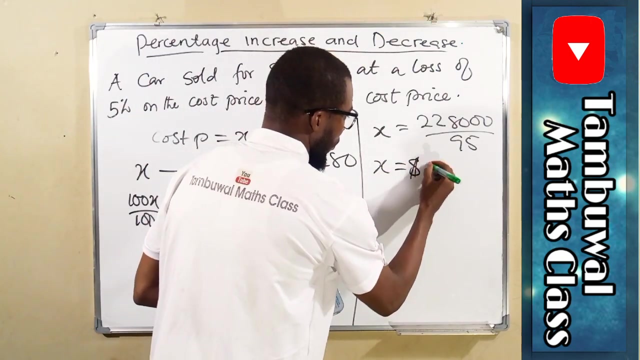 Therefore, x equals 2, 2,, 8, 0, 0, 0.. Divide by 95.. 228,000.. Divide by 95. We have 2,400 dollars. So this was the cost price: 2,400.. 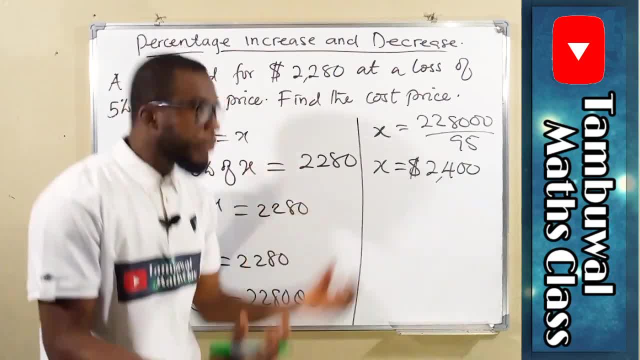 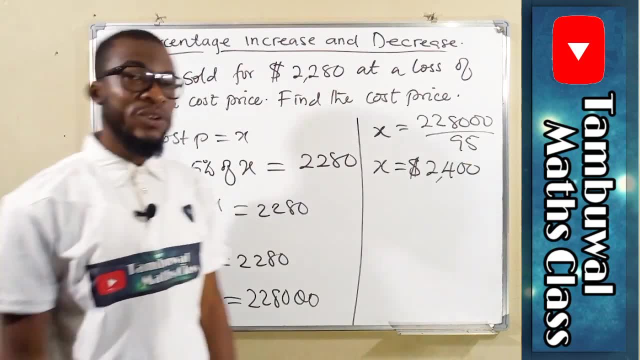 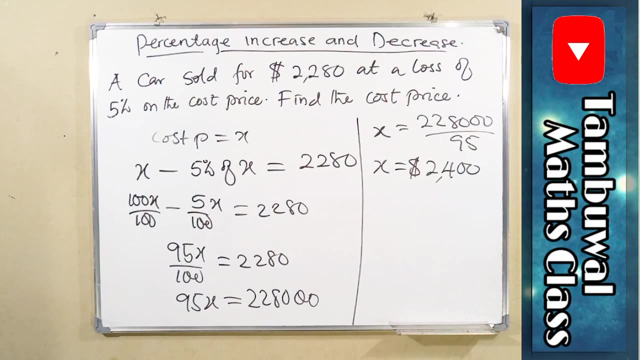 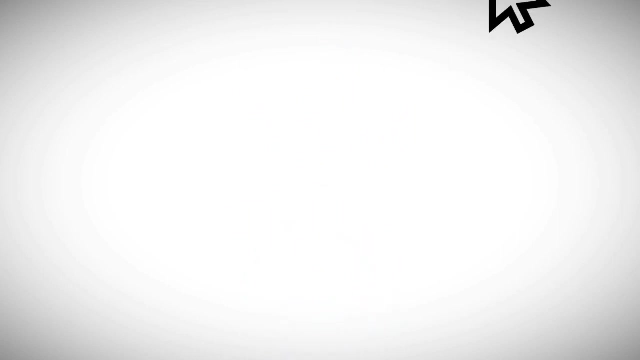 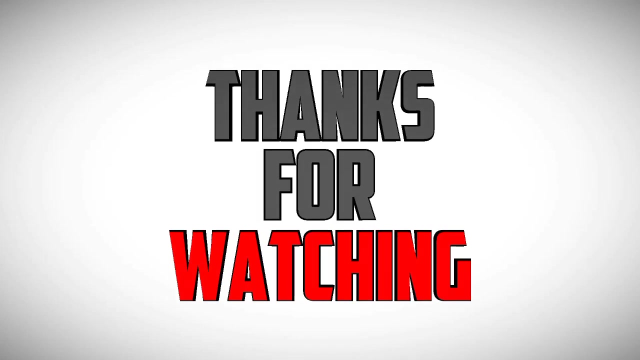 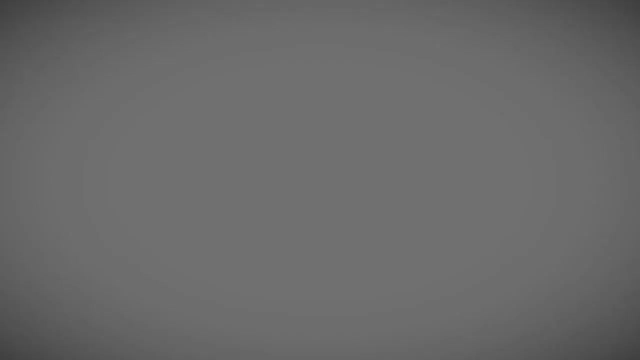 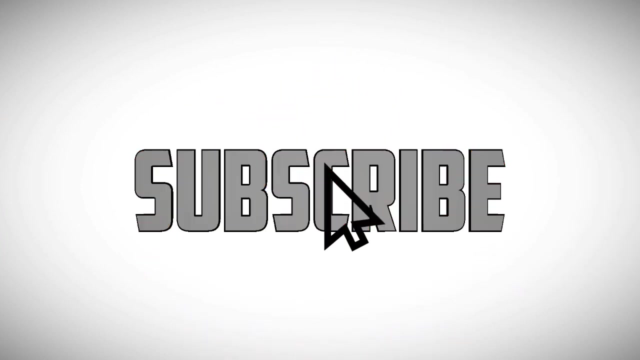 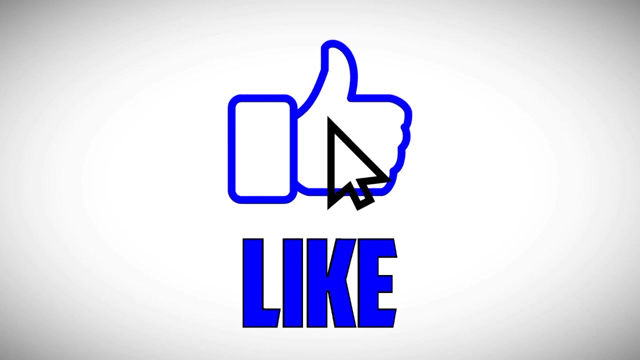 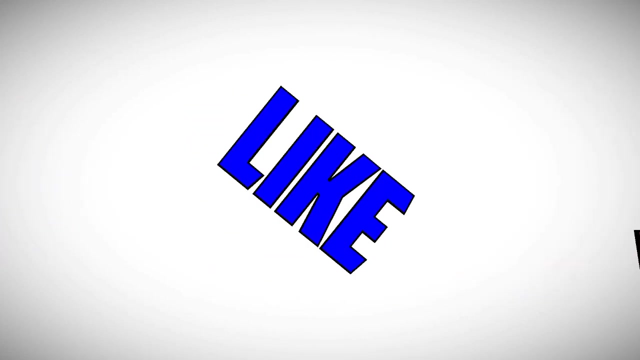 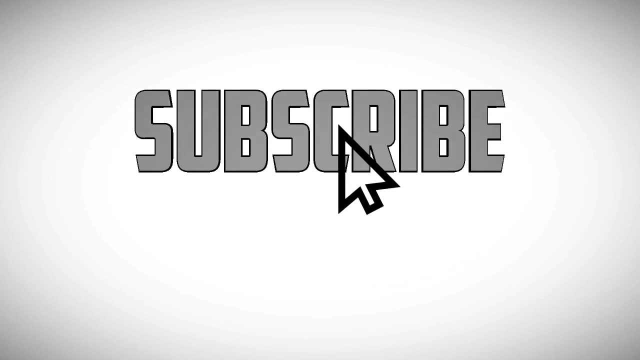 But later on sold at a lower price, which is 2,280.. So there is a loss. So this is all I have for you today. Thank you for watching. Do have a nice day. See you next time. Thank you. Thank you. 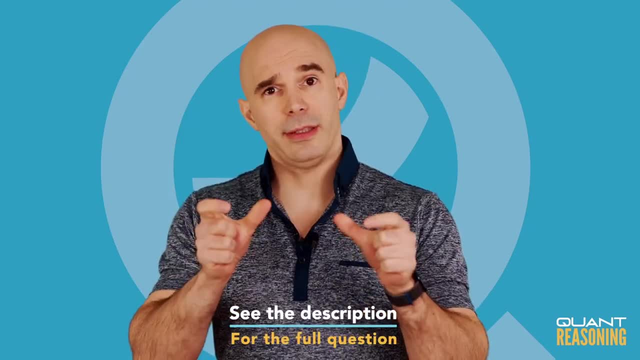 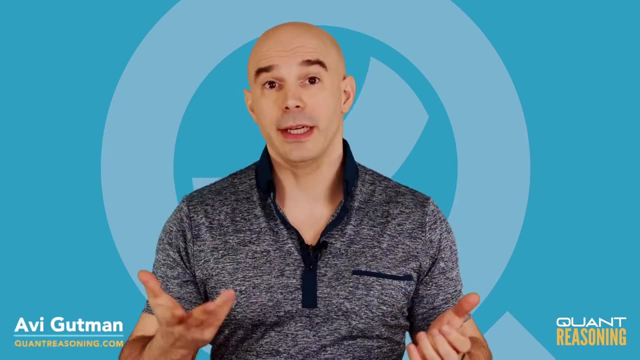 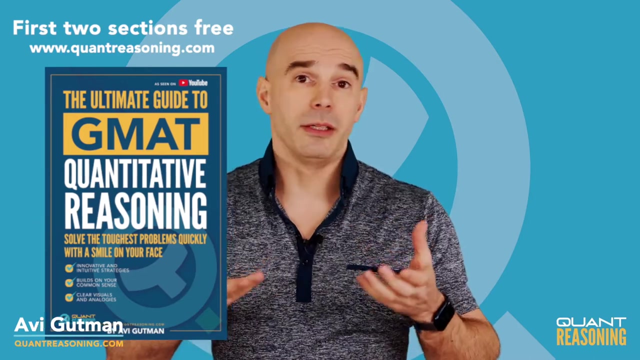 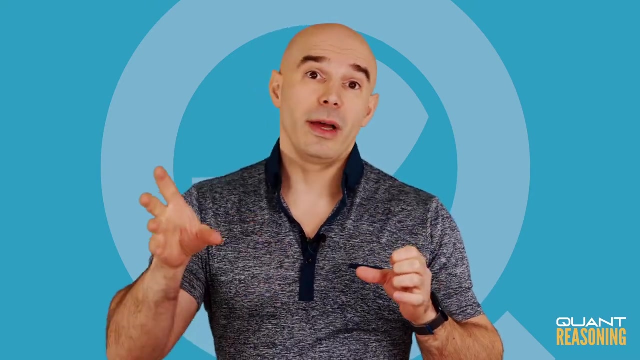 This question is talking about x and y, which apparently are basically exactly the same two-digit numbers, except in reverse order, so, for example, 38 and 83.. Now, as I explained in my book, for a question like this it's a good idea to just use a and b to represent the digits, and so we could say that x is 10a plus b and y would be 10b plus a. 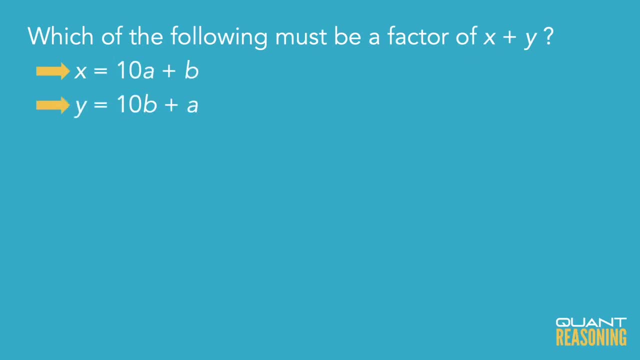 Now, when they talk about adding them together, you'd have 10a plus b plus 10b plus a, for a total of 11 of each 11a plus 11b, and since a and b are positive integers between 1 and 9,. 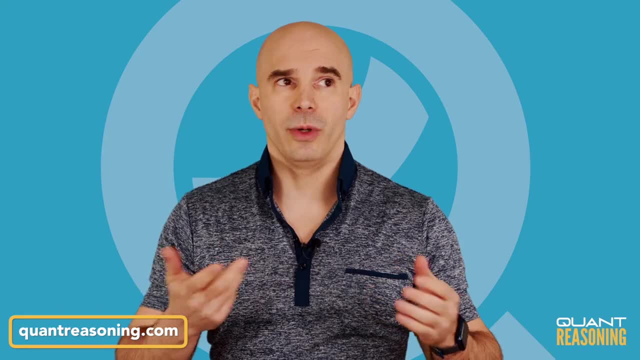 by the way, they can't be 0, because if one of them were 0, then one of our numbers would be a single-digit number, and we're told that they're two-digit numbers, so neither a nor b is 0.. 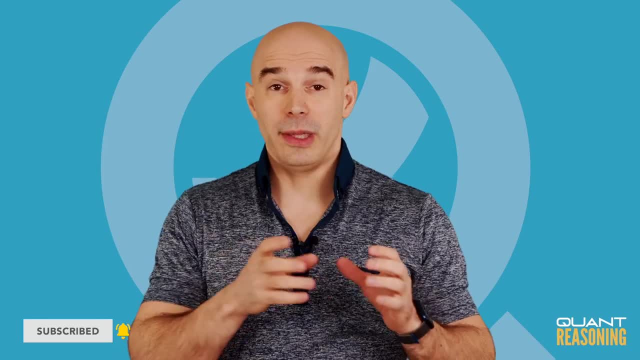 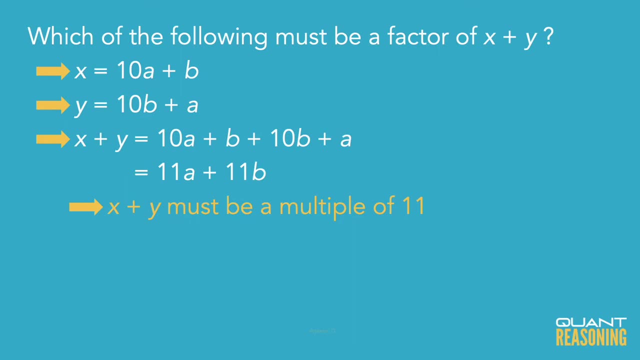 They're both positive integers between 1 and 9, and so 11 times the sum a plus b has to be a multiple of 11.. Based on that logic, I'm going to go ahead and pick answer choice D and move on to the next question.